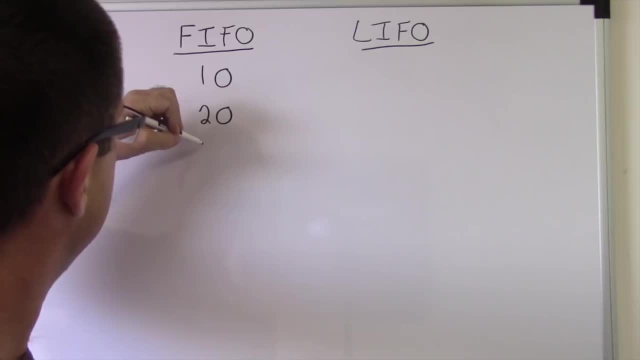 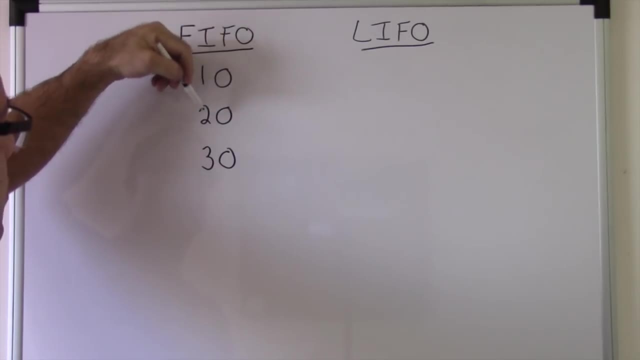 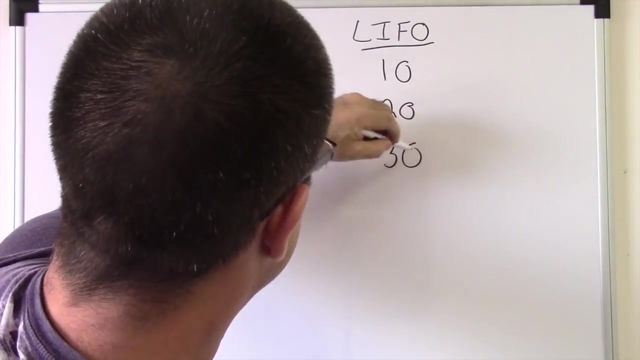 think the prices go down, But anyway. so $30, $10, $20, $30.. This is how you get the inventory, This is how you get your product. Okay, It's rising prices, We'll say you know. 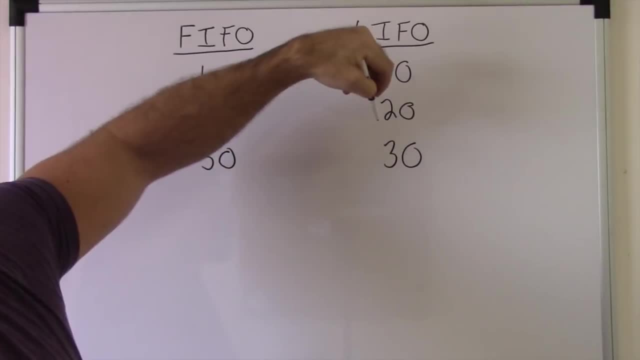 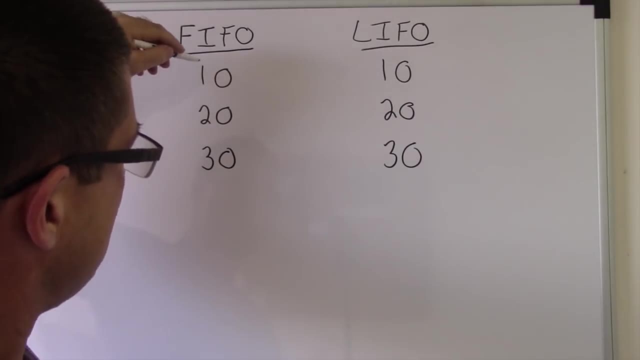 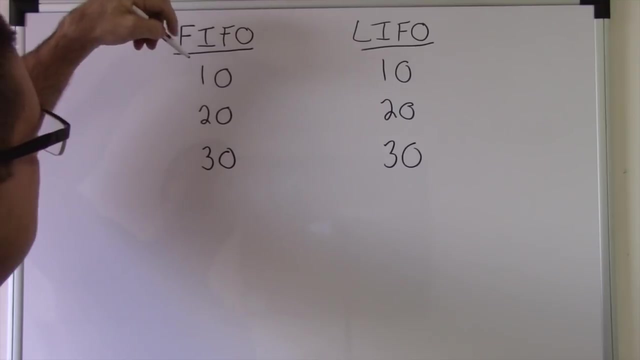 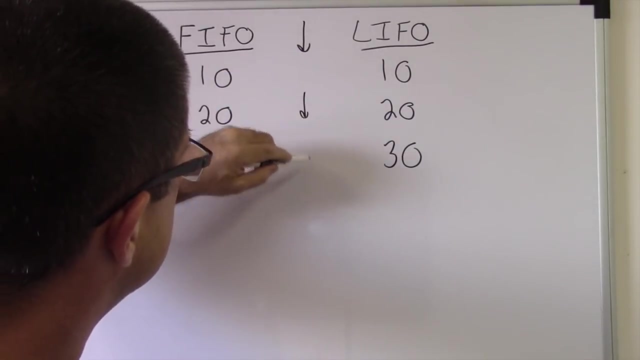 first batch is $10, second batch $20, third batch $30.. Okay, I kind of think of this as like a conveyor belt. All right, But anyways, first in first out. Okay, It comes from this way: Always in rising prices, You know right, Rising prices. So look first in first out. 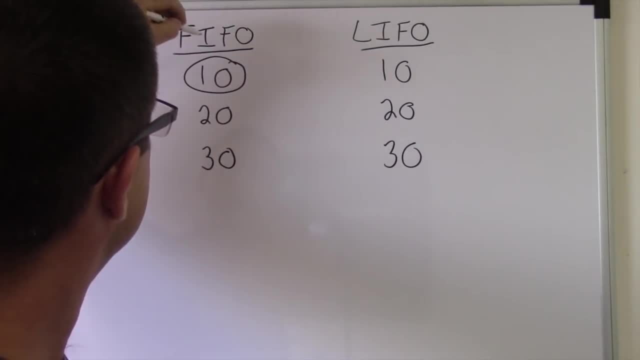 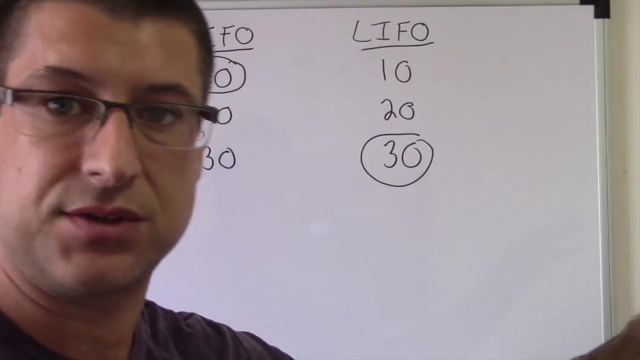 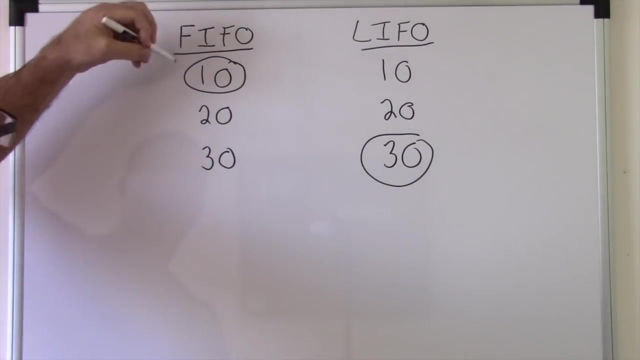 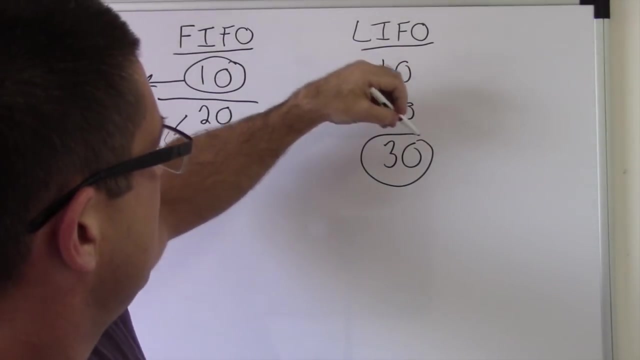 would be here. That's going to be the first out, Last in, first out There. So first out that they sold it, Sold it or last in. you know out means sold, So that's going to be your cost of goods sold. So look, that's COGS, That's inventory Right here. this is 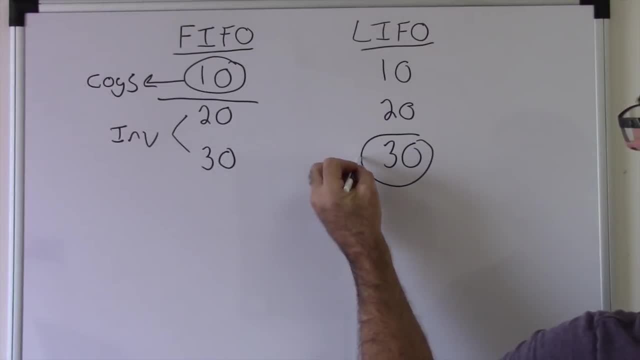 going to be, this is going to be your, this is going to be your, this is going to be your cost of goods sold. That's COGS Cost of goods sold, And here's going to be your inventory. All right, Got that. So if you do first in, first out your costs, your costs are going. 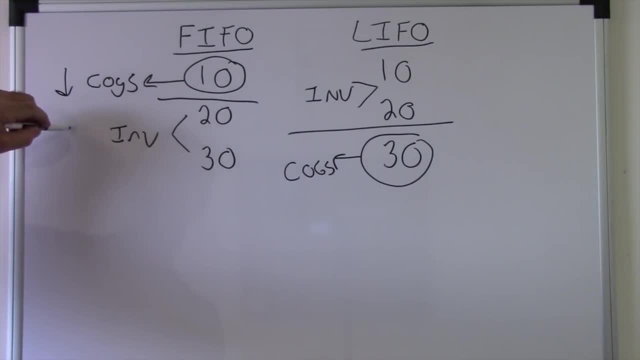 to be lower. Okay, Your inventory is going to be higher. Now what's that do to your income? If your costs are down, your income's up. They're inverse. What about on LIFO? If you do last in first out with rising prices, your costs?